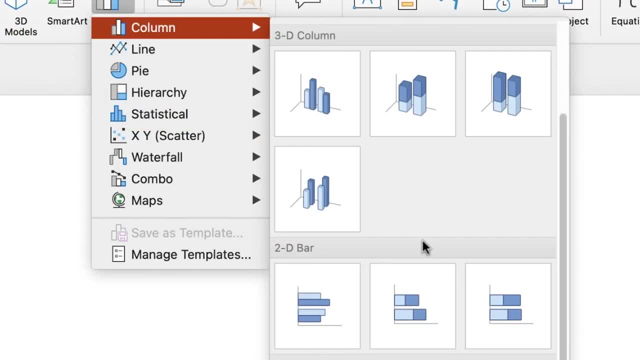 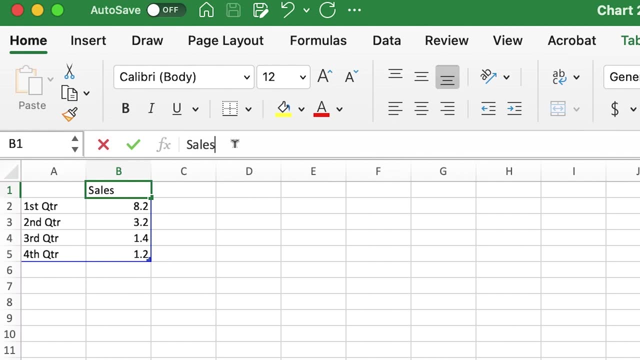 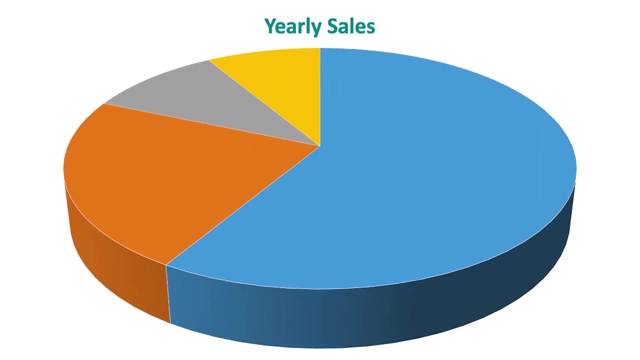 style your data in distinctive ways depending on what best suits your information. They display comprehensive sets of information, including numbers. Here are some key benefits of using a chart. Number one charts can show how data fits together. It's great for comparing portions to a whole. Number two charts also show how data relates to each other. 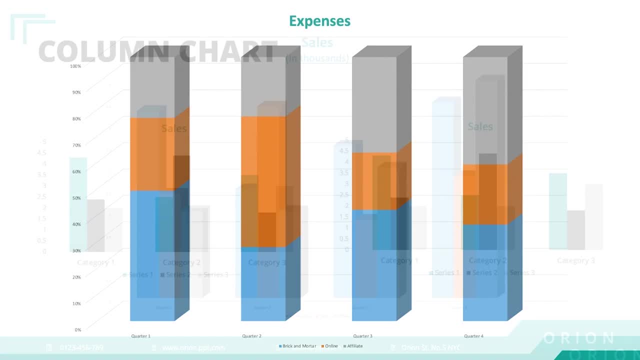 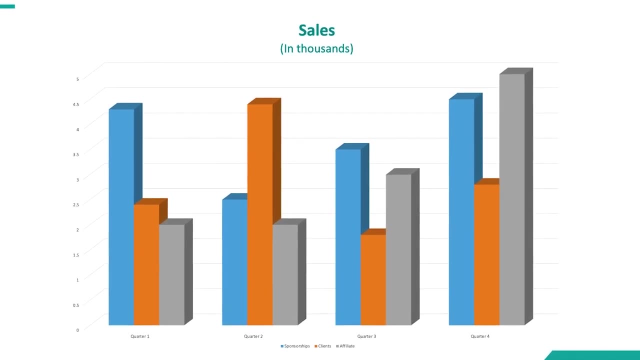 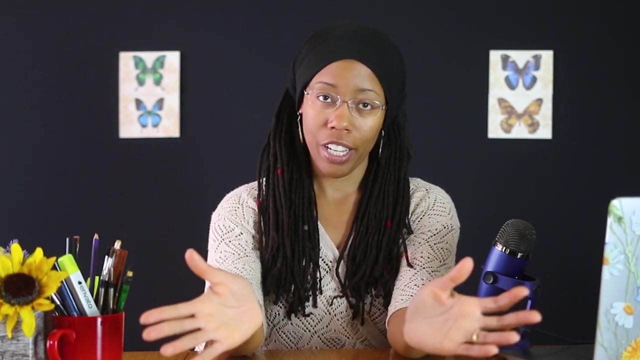 at a glance and allows you to compare them against each other. Number three charts also offer great flexibility. They let you show statistics, proportions and more. Now let's talk about when it's best to use a chart. The chart is great for flexibility and showing the big picture of your data. 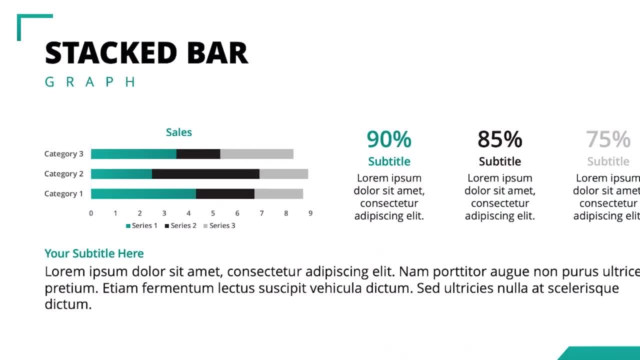 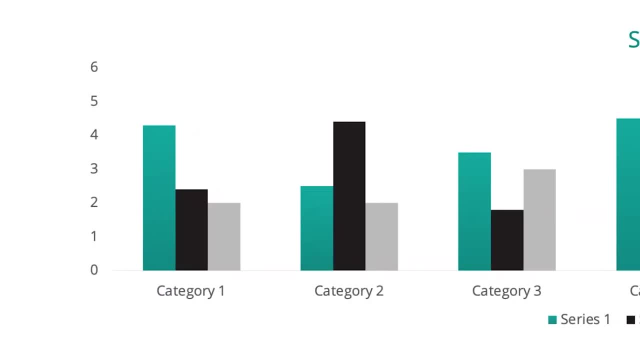 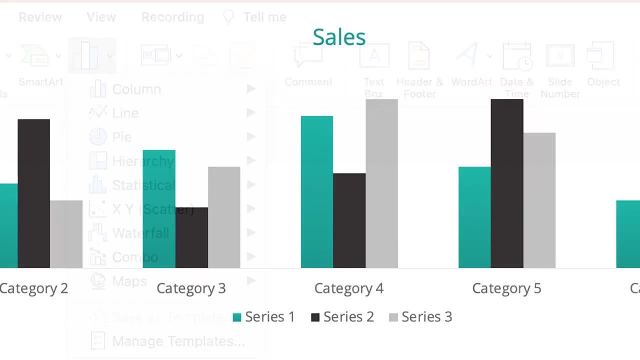 It comes in various shapes, styles and sizes. The types of charts you decide to use should reflect your specific goals for presenting your data effectively. Think about the overall picture you want your audience to take from your charts. So when do you use a chart? Let's take a look at some popular use cases for charts. 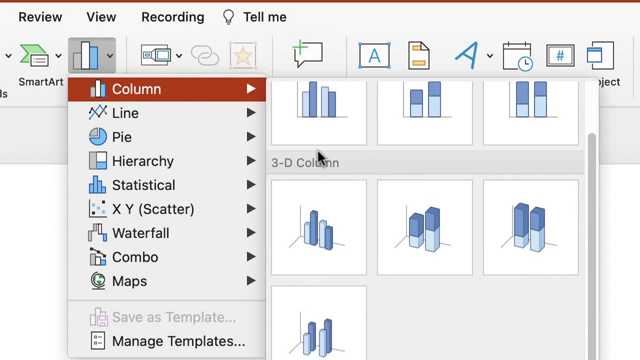 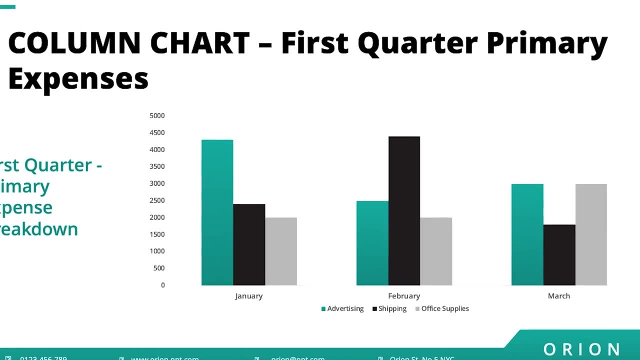 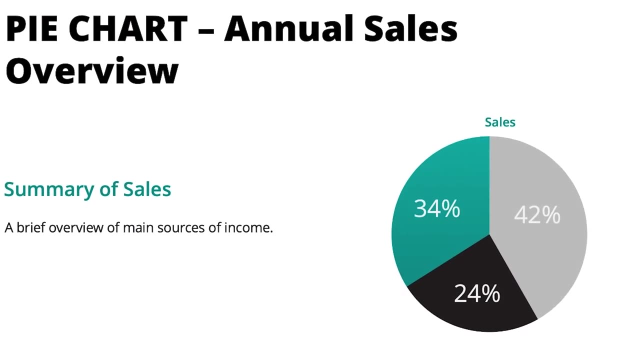 We have bar charts, also known as column charts, bars, and are handy for comparing variables against each other, as well as showing increasing or decreasing values. We also have pie charts. Pie charts are circular like a pie. They show how percentages of a data set compare to the whole. An example would be showing sources of companies'. 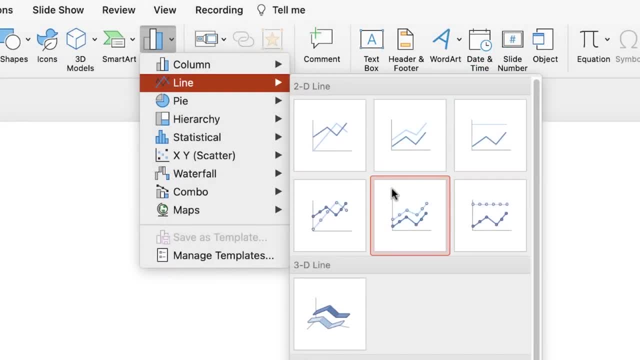 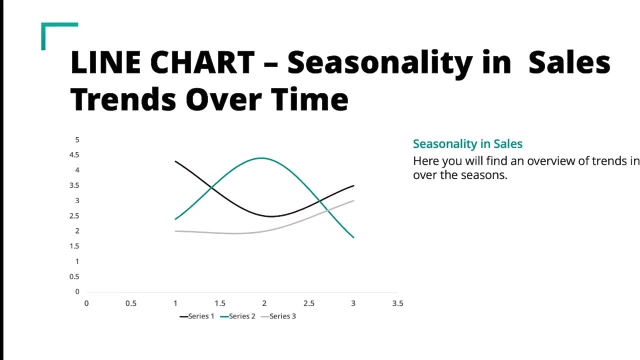 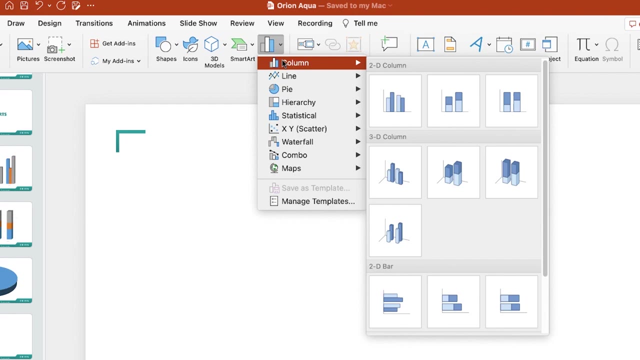 income sources. And we also have line charts. Their main component is a line or various lines that connect data points. They're great for showing trends. Consider the story you want to tell. Once you've decided the type of chart you want to use from your template, you can start. 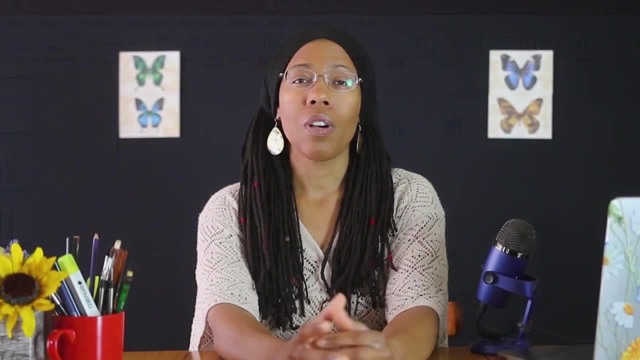 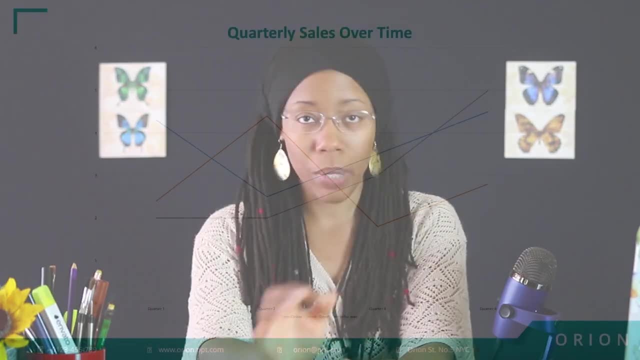 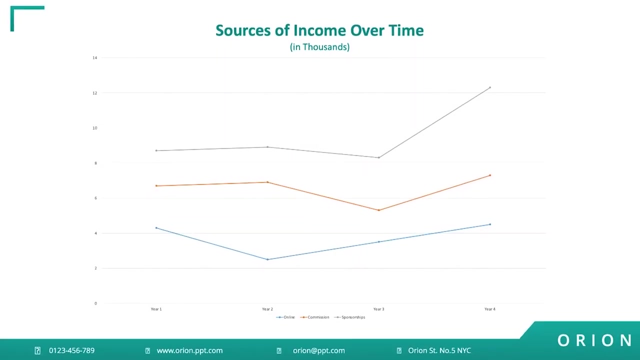 customizing it to your needs and data. Let's move on to graphs. So what is a graph? They actually have a more narrow definition and, specifically, they use data plotted on a grid. Although there are numerous types of graphs, they often use a grid representing various variables. They tend 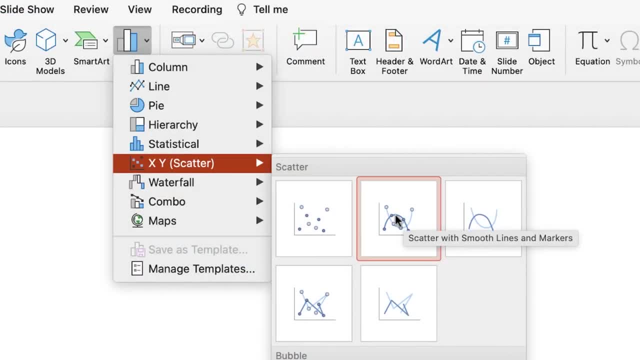 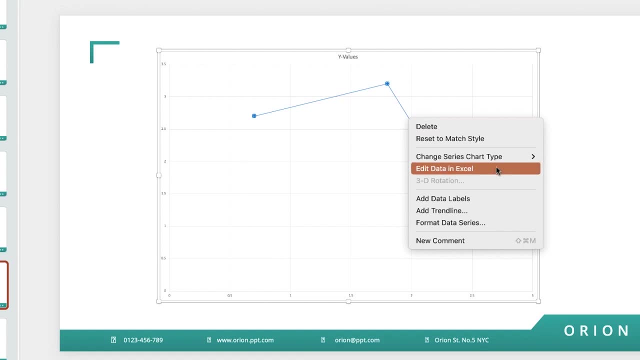 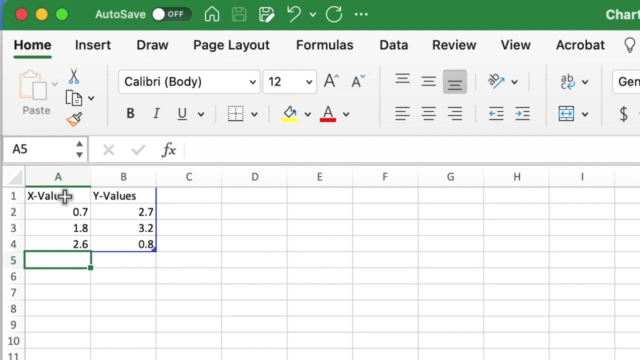 to focus on numbers to help you visualize your data. Graphs are perfect for numerical data. especially on a two-axis grid, It's a great fit for demonstrating data such as growth rates or comparable details. Graphs tend to be easy to digest and simple to understand Once you've labeled your axis, plotted your lines and put down your